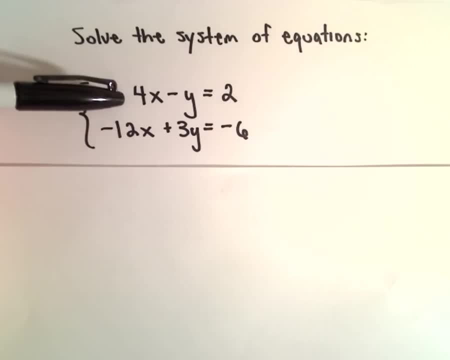 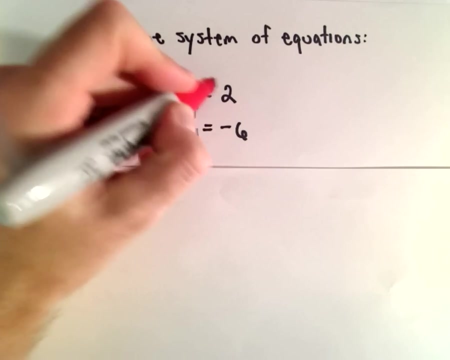 So I think you know, if I just had a positive 12x as my first term in my first equation, well then I could add: I would have 12x minus 12x. the terms involving x would cancel, So to make a 12x appear. what I can do to my first equation is I can simply multiply both sides by 3.. 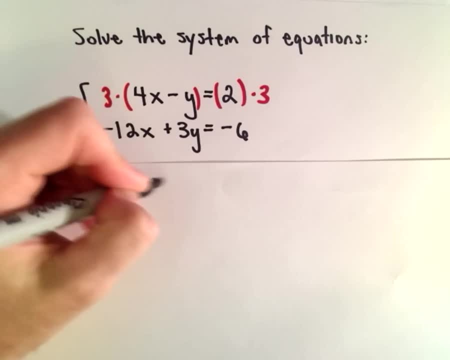 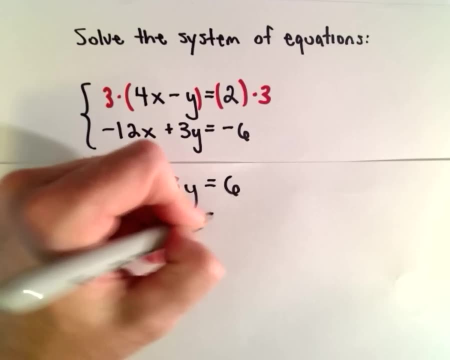 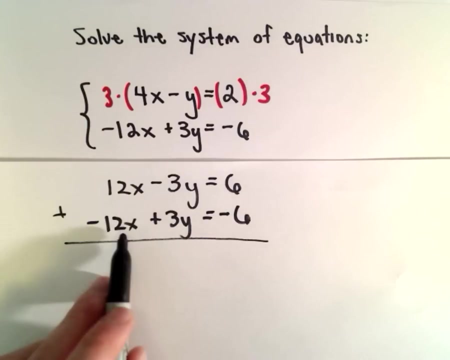 Well, if I do that, I'll get 12x minus 3y equals 6, and then we have negative 12x plus 3y equals negative 6, just our original second equation. Notice: if I add these two equations, I'll get 12x minus 12x. 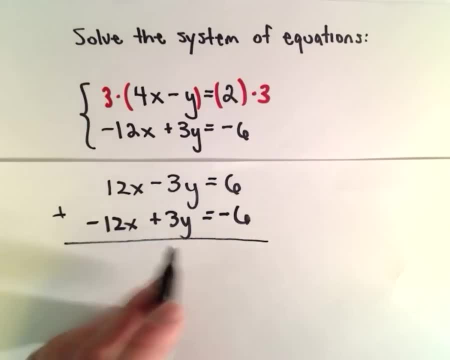 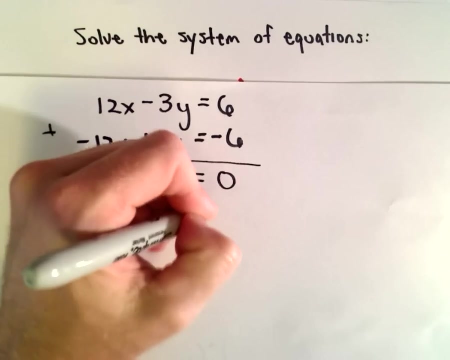 I'll get 0x negative. 3y plus 3y is 0y, so we're left with 0 on the left side. On the right side, we have 6 minus 6, which is 0, and what this tells me is we have infinitely many solutions. 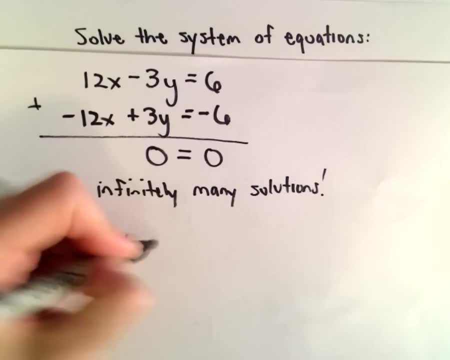 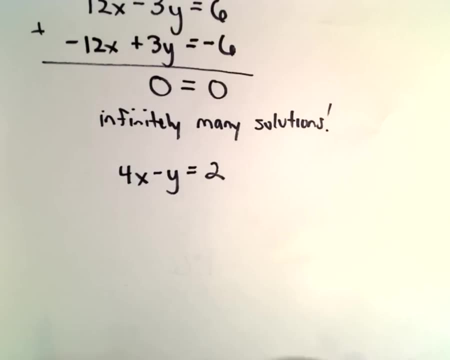 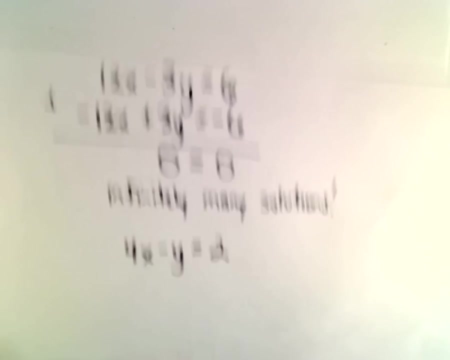 So if you actually want to write your solutions down to sort of give a a generic sort of form- people sometimes ask for this- What you can do is take any one of your two equations. I started with the 4x minus y equals 2.. 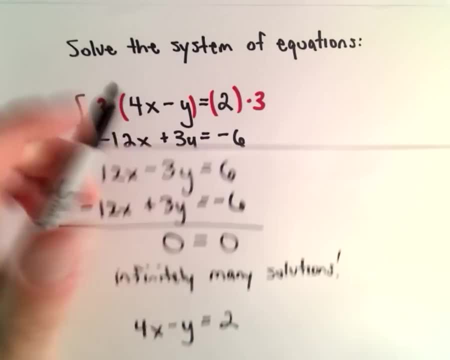 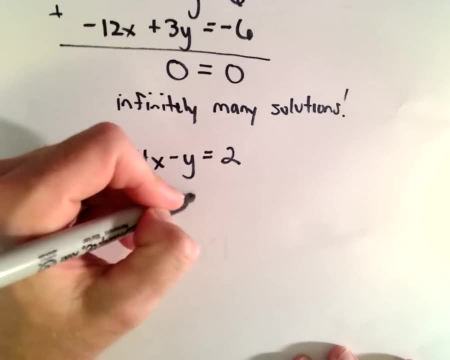 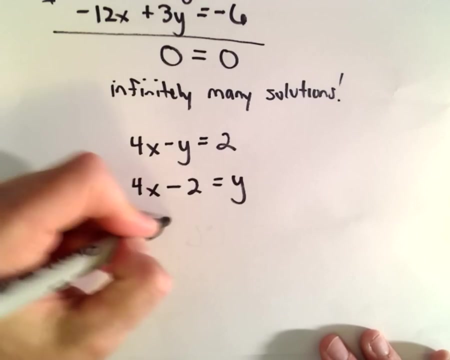 I started with my equation. before we, you know before we multiplied everything out: 4x minus y equals 2.. I'm going to solve for y, So I'm going to subtract the 2 to the left side, I'm going to add y over. and now the idea is we can say: let's let x equal some constant k. 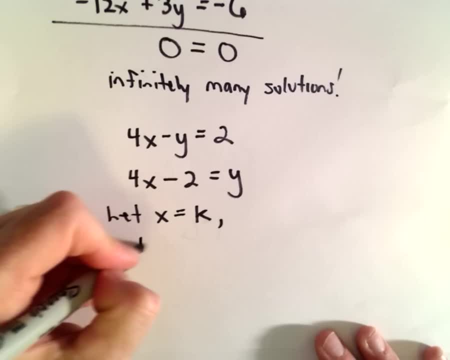 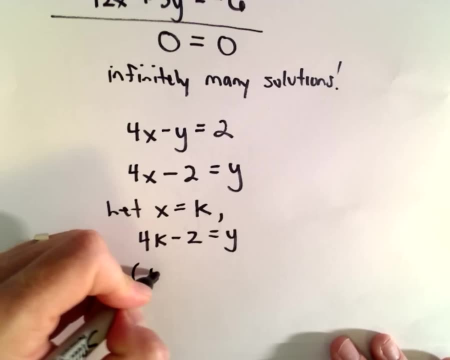 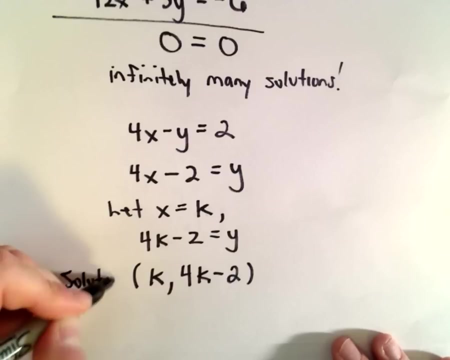 well, if we do that, then y is going to equal 4k minus 2.. So we can say our solutions are of the form k comma, 4k minus 2.. So the idea, the idea is pick your favorite value for x and then do 4 times that number minus 2, that'll give you the y value. 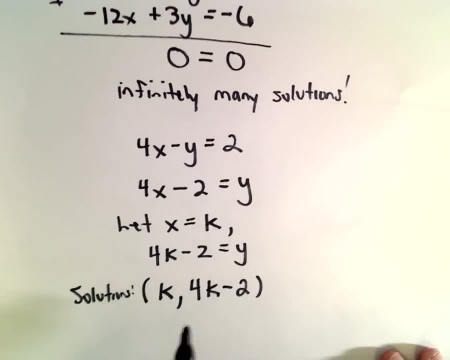 and that's the way that you can actually find your solution. You can find specific, specific pairs of numbers that satisfy the original system of equations.